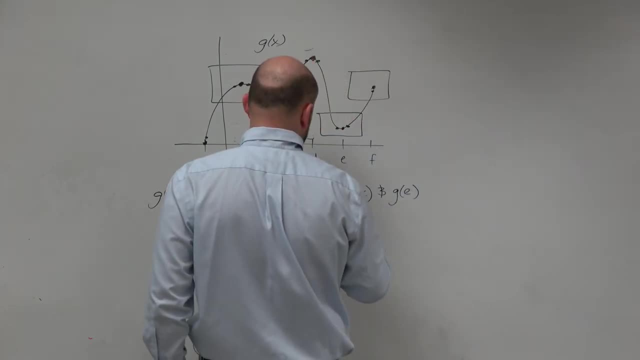 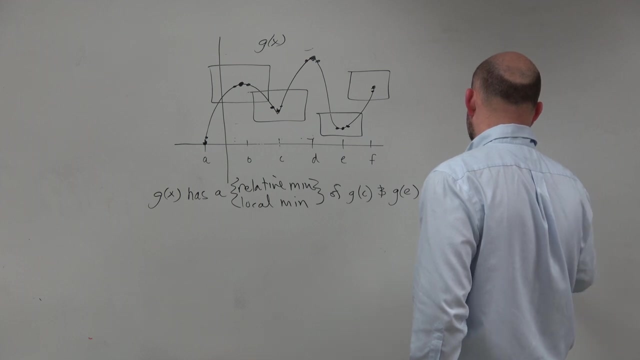 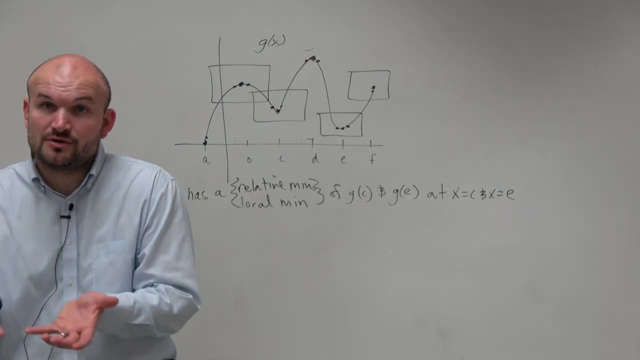 Oh, of, sorry, of g of c and g of e, at x equals c and x equals e. So would you guys agree those? we're talking about the global, the minimum, but then also where those values occur. Yes, Okay. 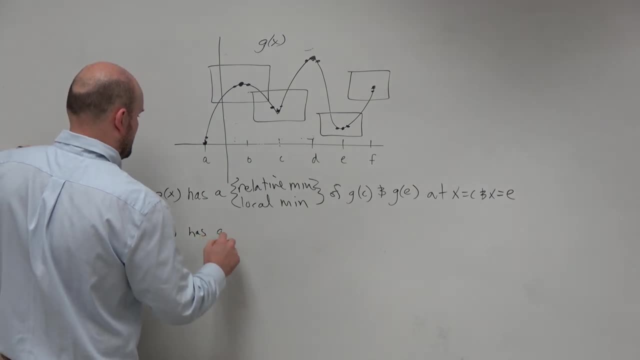 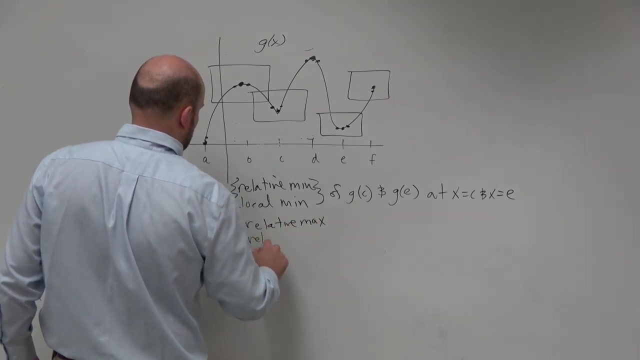 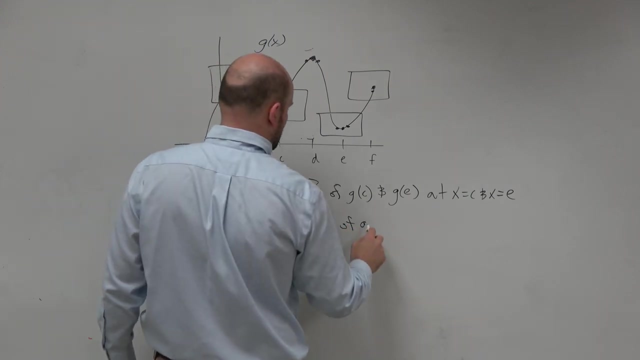 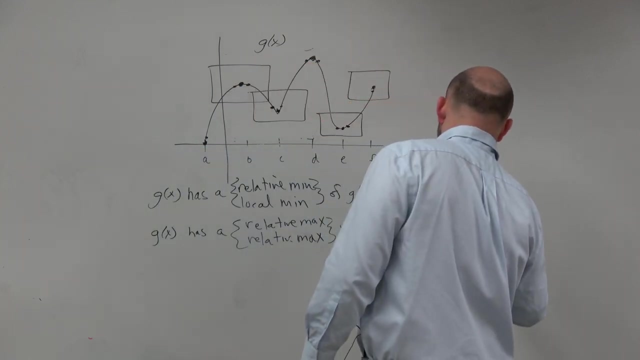 And then we could say: g of x has a, a relative max and a relative min of- I'm sorry, relative max. what was this? g of d, no, sorry, relative min. at g of b, of g of b and g of f, at x equals b and x equals f. 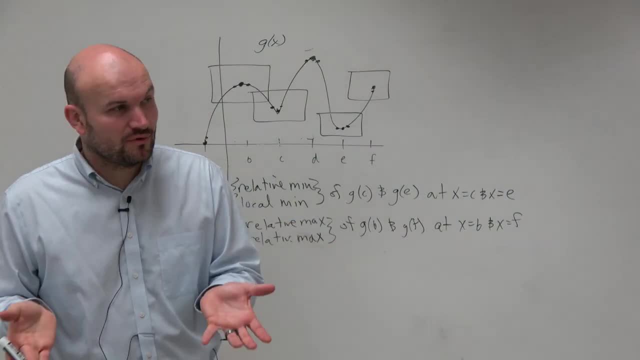 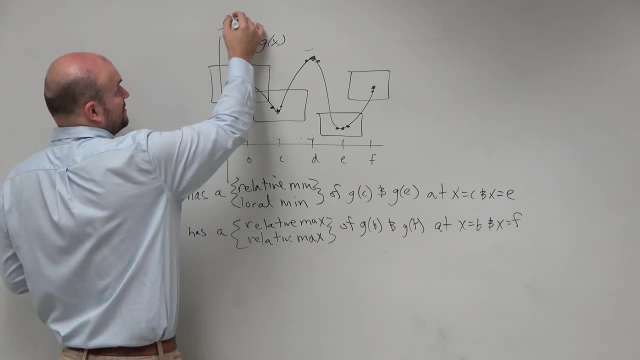 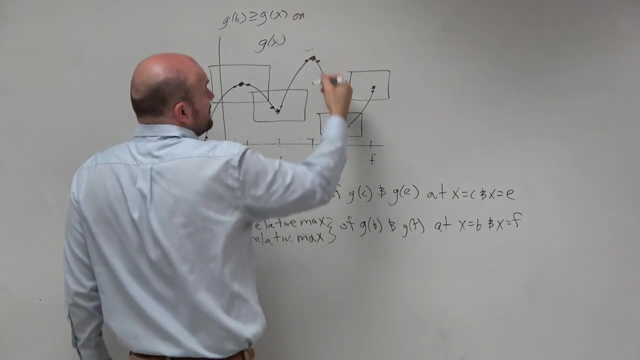 Okay, Now, When we're talking about the relative min and the relative max, what we're? it's the exact same thing, like. the reason why this is a maximum is because that g of b is greater than or equal to g of x on a given interval. 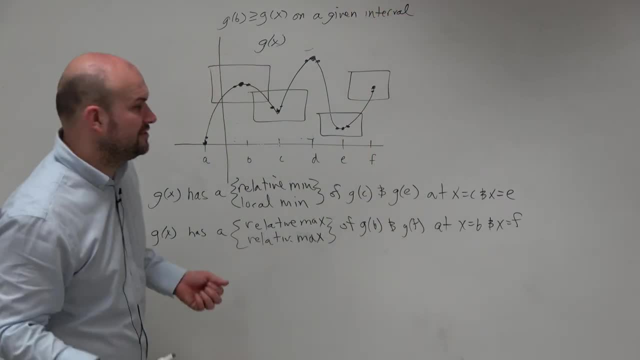 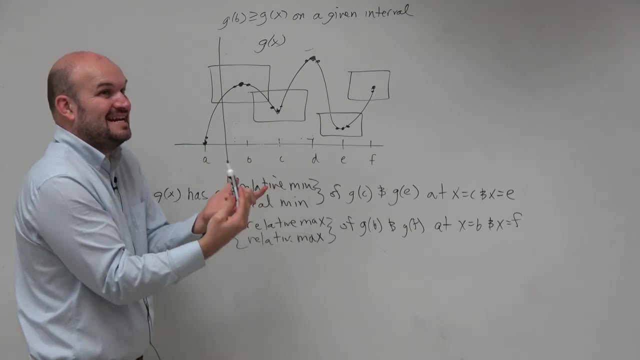 And now, like what would that interval be? You could say that interval is like between a and c, right, Don't you guys agree with me, Like so, As long as it's on any given interval. a lot of times we just call it interval i. 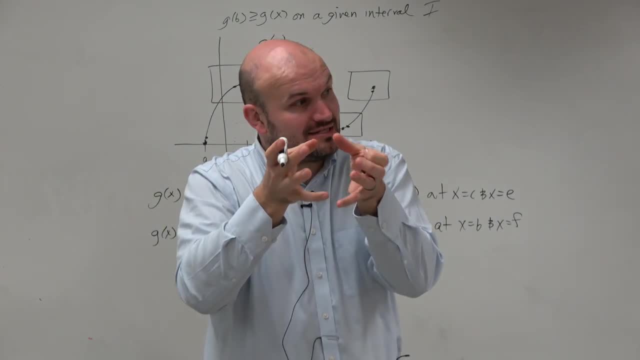 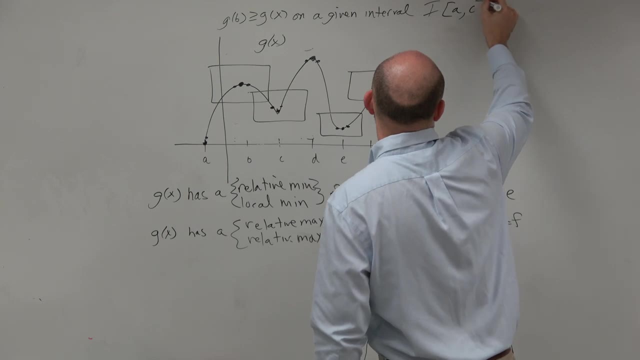 because if you have an interval and you could say that like that value is, like your max is your absolute maximum in that interval, then it's a relative max or min And like. for example, you could just say like from a, you know, to c. 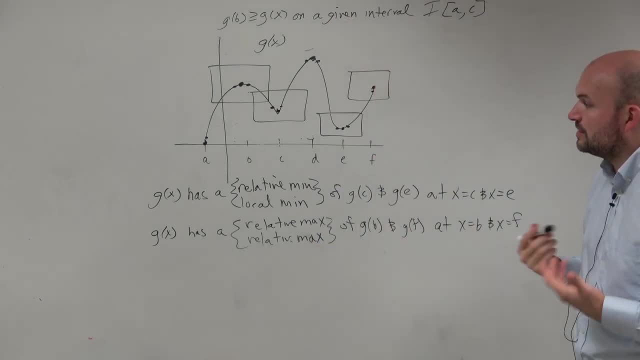 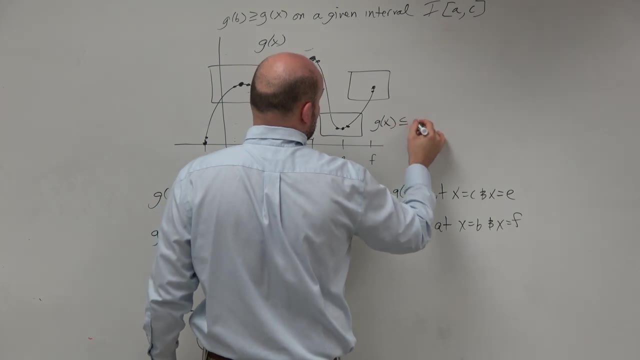 which is going to be producing your, your relative, relative maximum, And that's going to be occur. like the same thing for g of e. We could say that, you know, g of e is less than or equal to g of x. 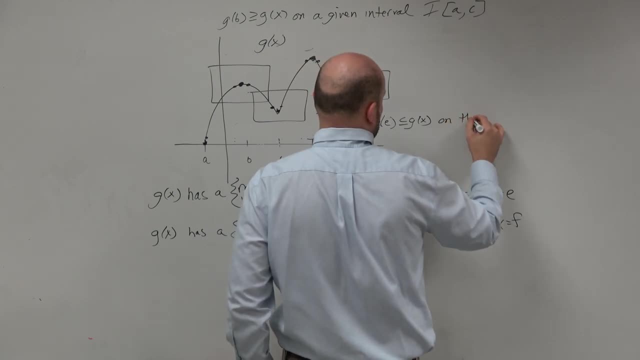 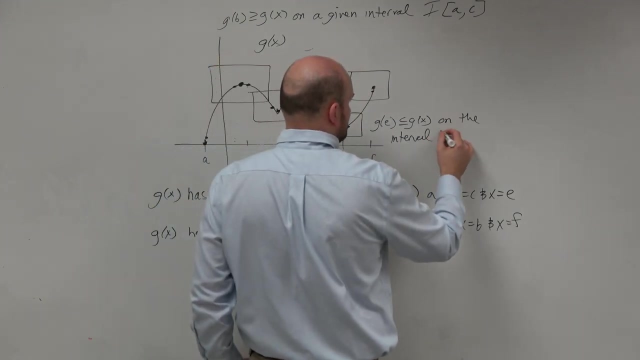 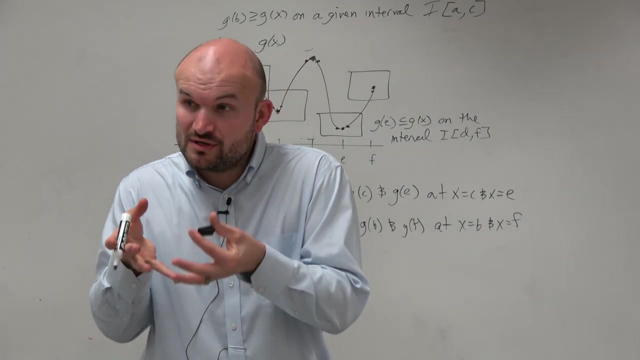 On the integral, you know i, which is, let's say, from d to f. You know. so, if you can determine an interval and that value is the lowest term, then that's important. Now, the next thing I want you guys to look at, which is a? really, really really.